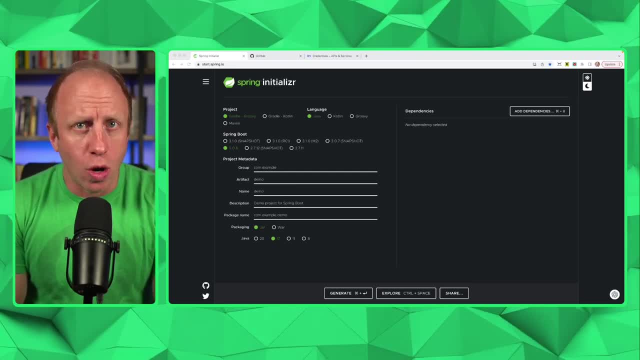 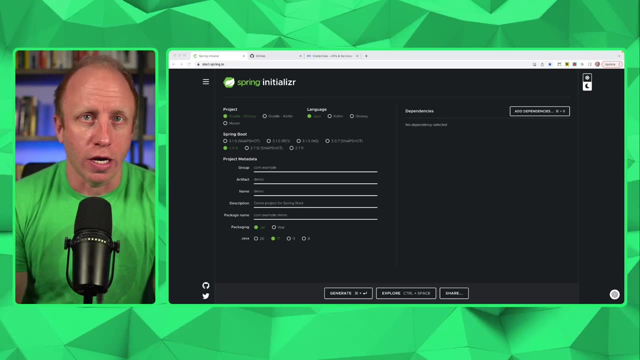 What's up friends? Dan Vega, here and today we are talking about OAuth 2 logins in Spring Security. So if you have an application and you want to provide a way for users to log in, you can have them log in via form using something like a username and password. 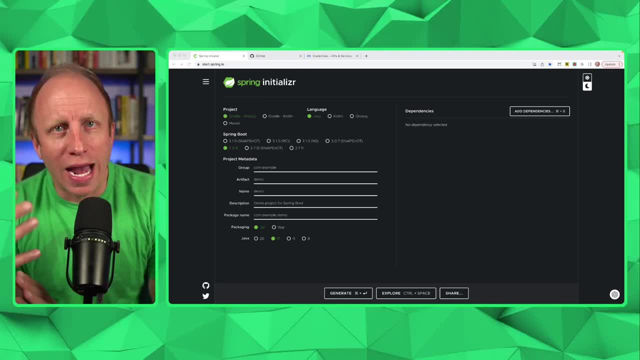 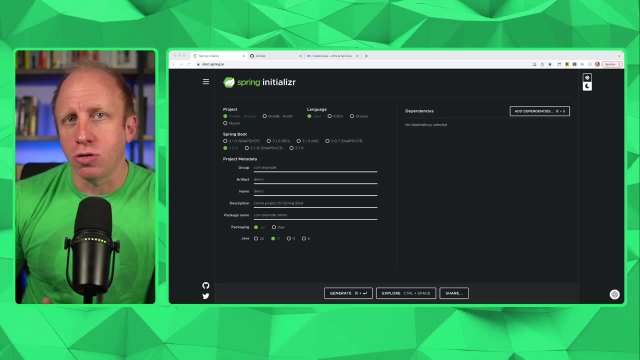 maybe an email address, But if you don't want to have to have your users register on your system, you can have them log in via some social login like GitHub, Google, Twitter, whatever the case may be. That's what we're going to look at today. We're going to use Spring Boot, Spring Security. 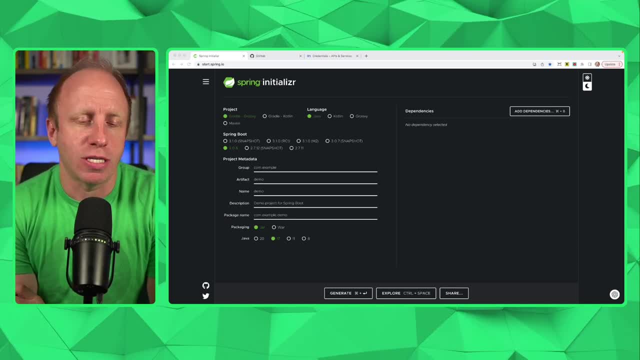 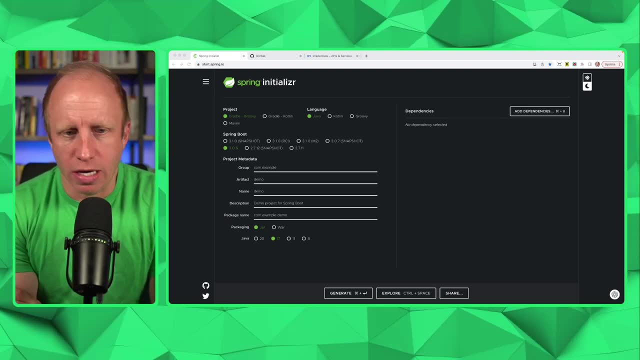 and the OAuth 2 login functionality that's built into Spring Security to make that happen, And it's actually really easy to do. I've gotten a lot of questions about this lately so I thought we'd just jump right in. Here I am at startspringio. I'm going to create a new project. 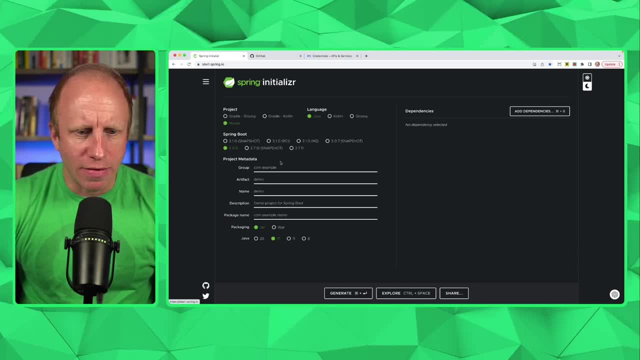 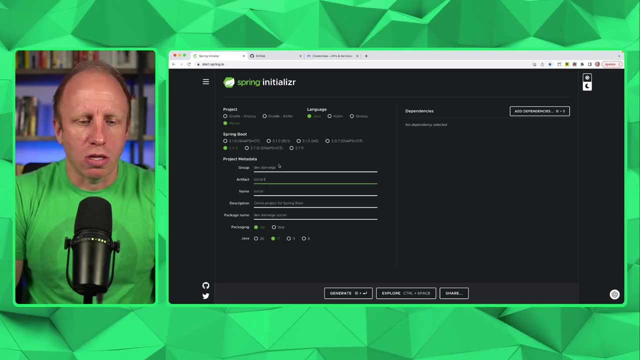 I'm going to select Maven as my build tool, Java as my language. I'm going to change that group to devdanvega. We'll call this a social login, if I could spell Dan, And then we'll choose Java 17.. And we're going to need a couple. 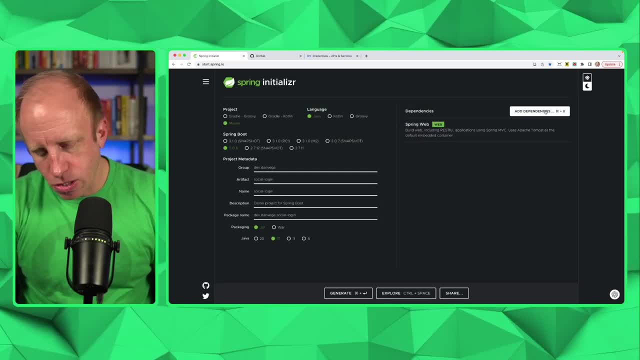 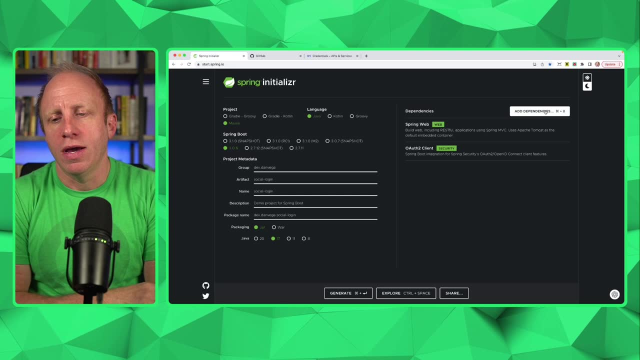 dependencies. So I'm going to choose web. I'm also going to choose the OAuth 2 client. This will bring in Spring Security as a transitive dependency, And so we'll have everything we need. That's really all we need to get started. So what we're going to do is we're going to generate that. 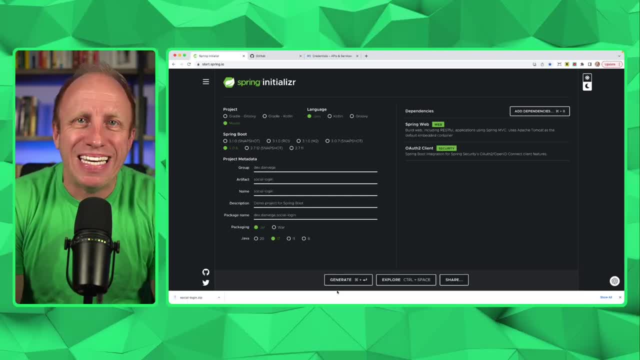 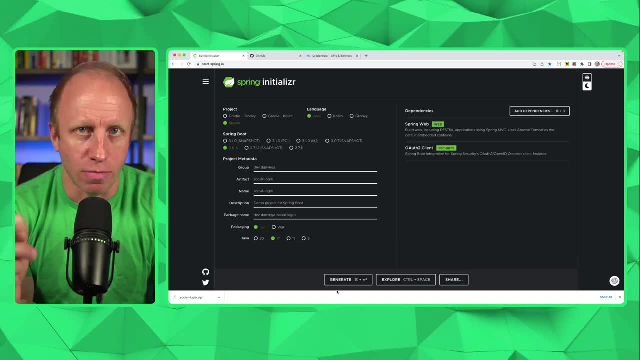 project. It's going to download a zip. I'm going to open it up in IntelliJ Ultimate IDEA- That is my favorite IDE, But you should be able to download that project And then we're going to open it up in whatever text editor or IDE your most productive in. What are we waiting for? Let's. 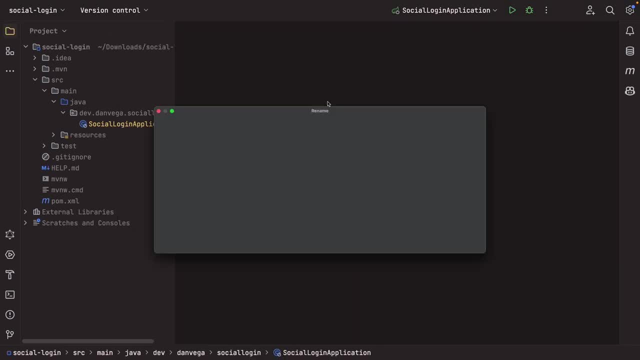 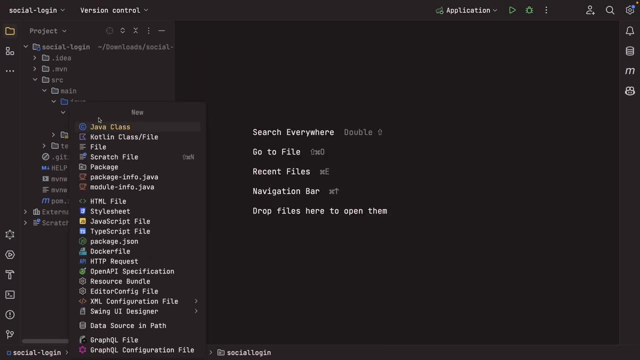 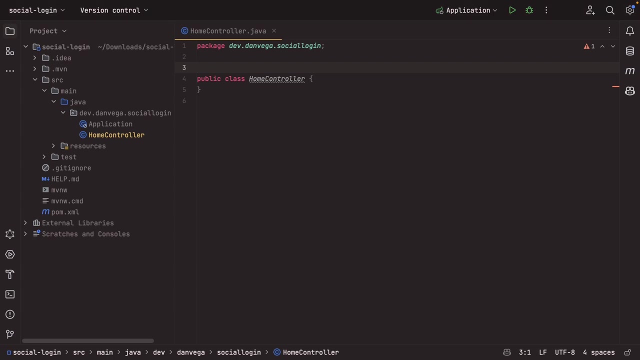 write some code. All right, I'm going to get started by renaming this to application And we are good to go. So the first thing that we need is we need a controller. So I'm going to create a new Java class called home controller. I basically want to set up a route that is public and a route. 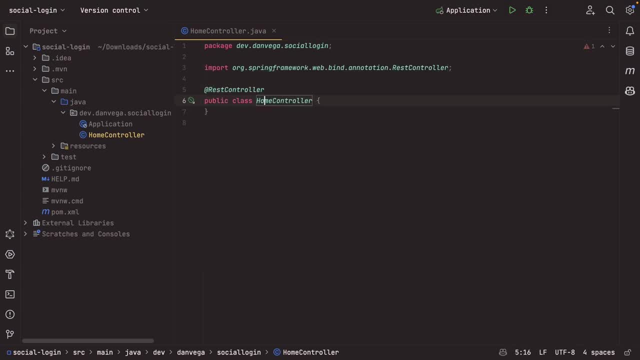 that is private. So I'm going to mark this with rest controller And then we'll create a couple here. One get mapping for the route context. So slash, This is going to be public, string home, This is going to return hello home, And that is all for that. And then we'll need a secure mapping. 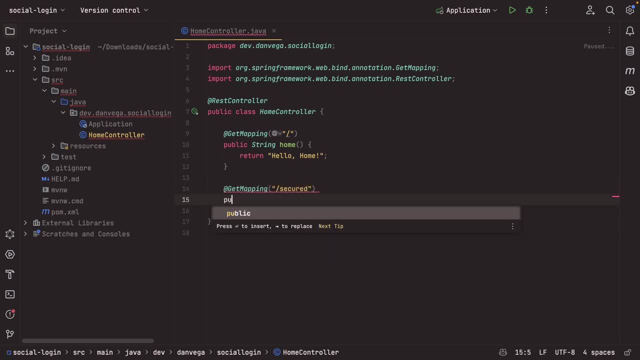 So we'll say slash secured, And this will be public string secured, And then this will just return: hello secured, And that is all we need. We'll need to set up some configuration where anybody can get to home, But if you log in or if 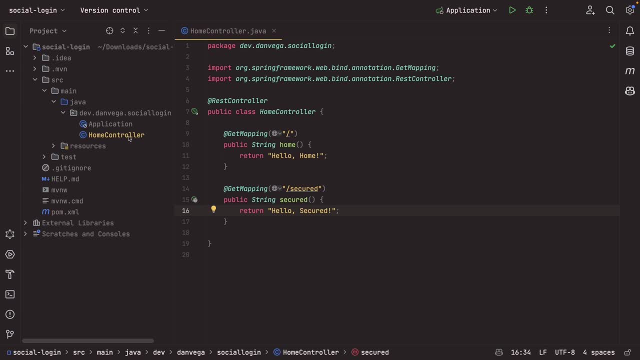 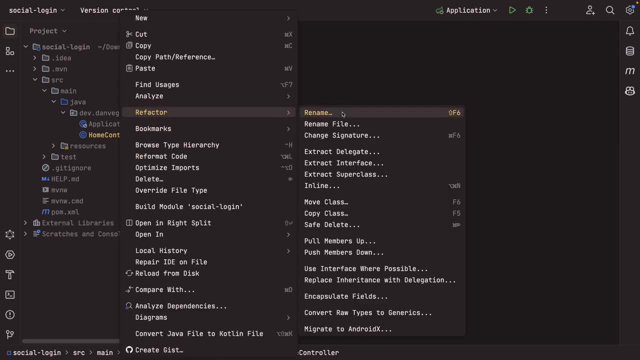 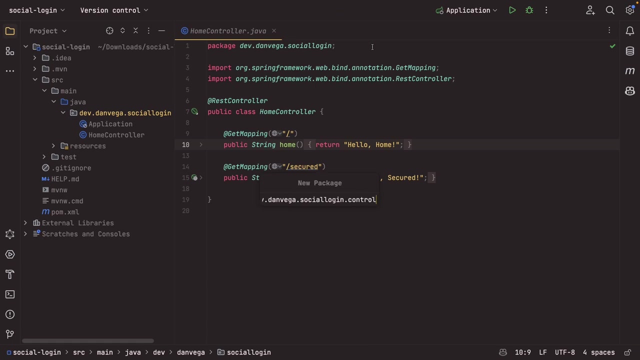 you hit at secured, slash secured, then you will need to go ahead and log in. So just to make sure everything is working. I wanted to put that: Why did that not go in a package called controller? Come on, Dan, All right, So we refactored that. Now I can go ahead and run. 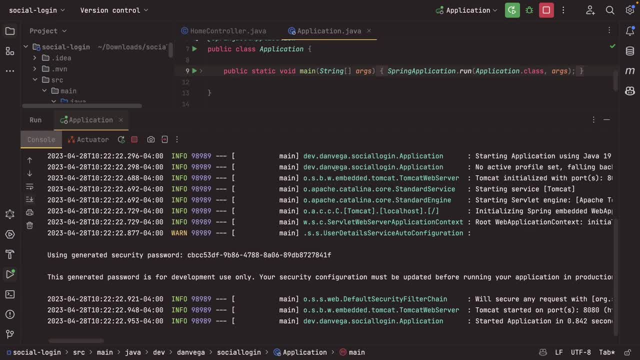 And because Spring Security is on the class path, we basically get a default user and a default password. If this is your first time using kind of Spring Security, you go ahead and check out my channel. There's a bunch of videos on the topic. But we have this randomly generated password that 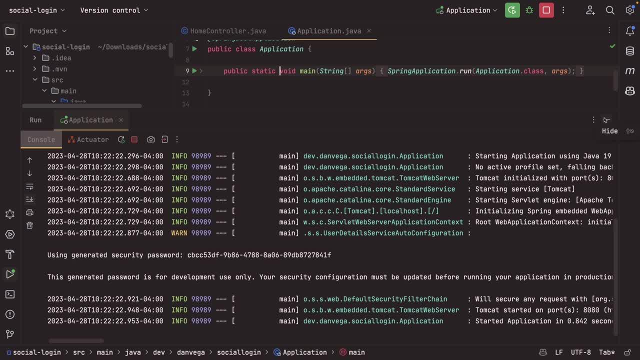 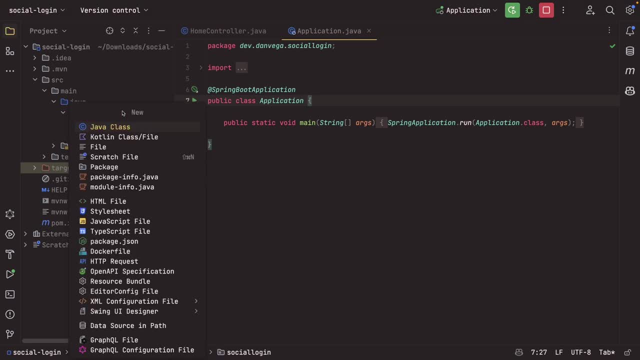 we need to log in with, And then everything is secure by default. So to change this, we want to override our security configuration. So we're going to create a new Java class. We'll call this security config, And then we're going to create a new Java class, And then we're going to create a. 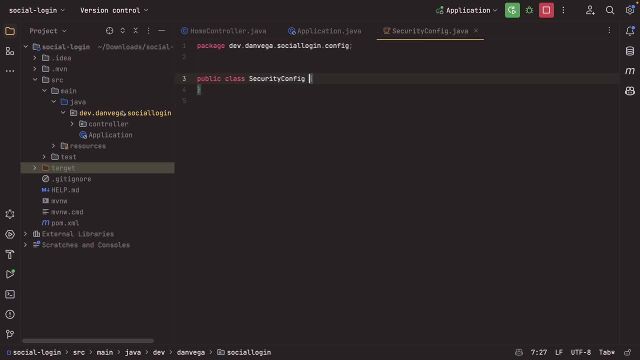 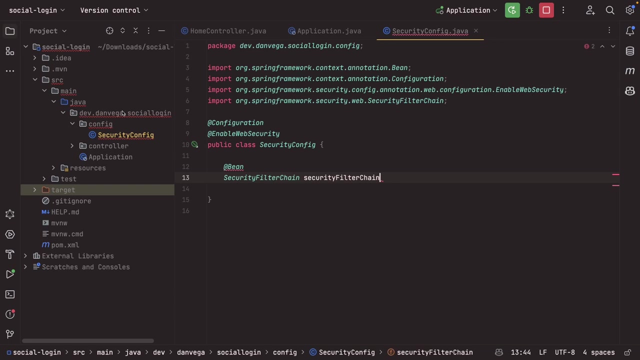 security config And we'll put it in the config package. So security config, And we'll mark this with at configuration, at enable web security. This will get us going. And then we need to create a new bean of type security filter chain. We'll call this security filter chain. This takes in. 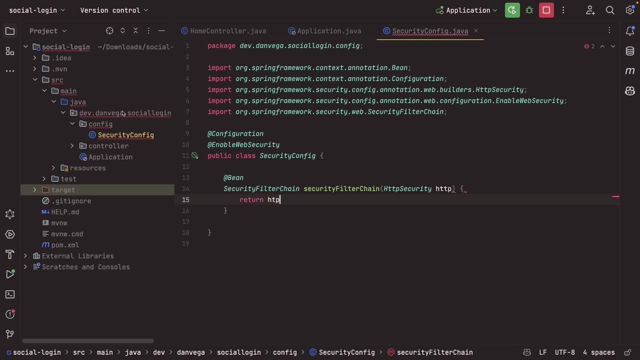 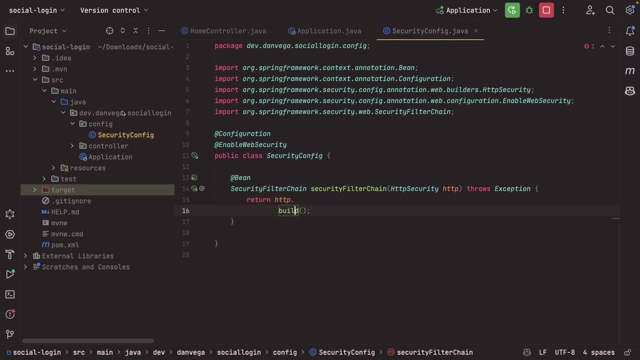 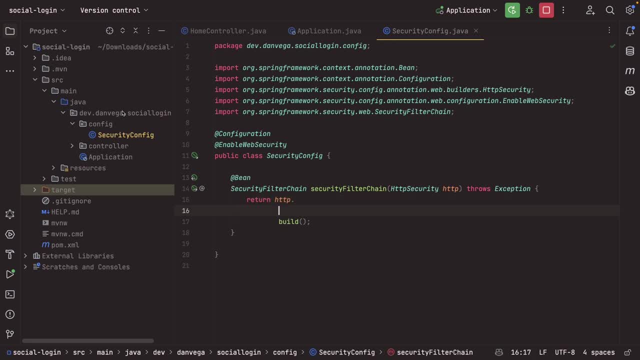 and add next to it, And then we'll go ahead and add next to it, And this will go ahead and add next to it, And we are ready to go. So now we need to configure Spring Security, All right, And so we'll use. 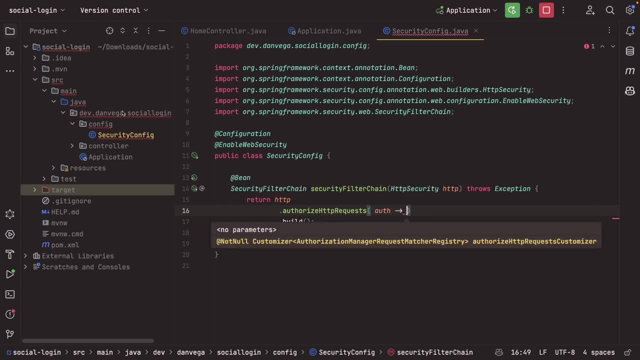 authorize HTTP requests and the Lambda DSL here And we'll say auth dot request matches. So we'll say for our home route that anyone can get to that. We'll say that And then we'll say any other request. I want you to make sure that they are authenticated. Now how are you going to log in? 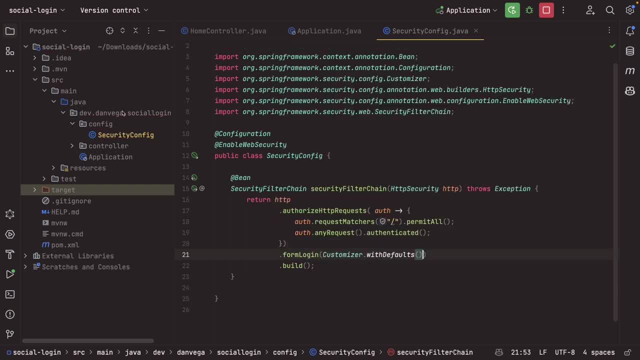 so we can provide a form log in with some defaults And that will. let's go ahead and import that static And that will give us a form login. So now, when we visit slash secured, the user will have to log in with their username. 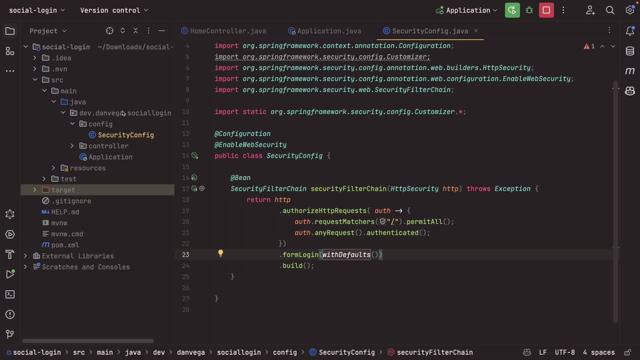 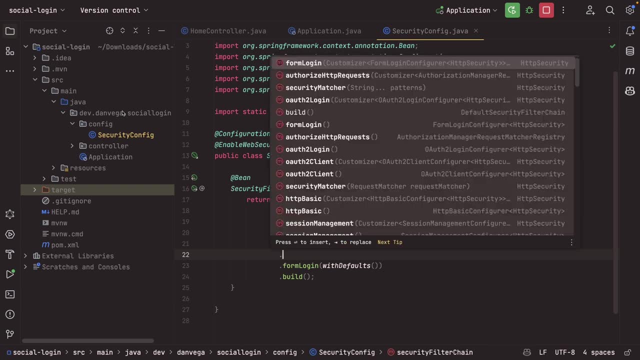 and password to be able to view that. But we don't want to just provide a form login. Maybe we want to provide OAuth 2 login. So how do we do that? So first off, we can say OAuth 2 login. We can. 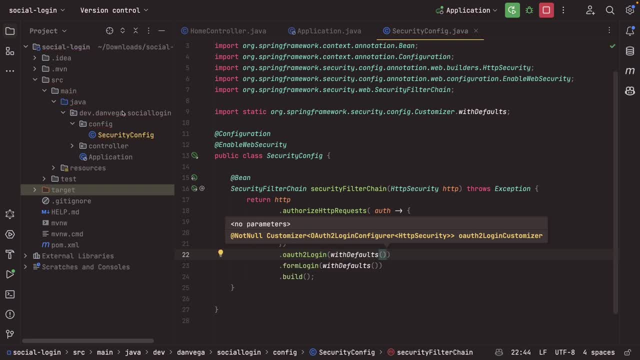 also pass the defaults to that And that's all there is to it. That is our setup there. We need to create some properties in applicationproperties to say what OAuth 2 clients we're going to support or what OAuth 2 providers. So if I go into applicationproperties I can fill in some. 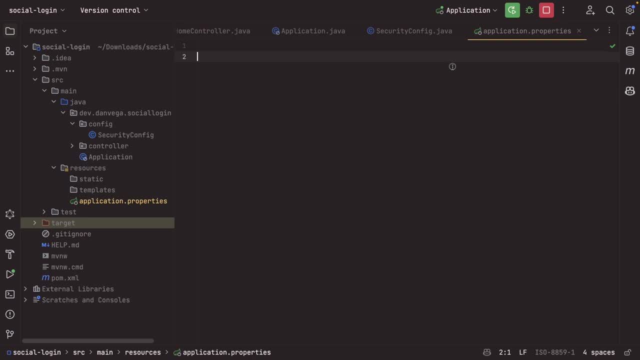 properties So I can set up. let's just say, for this example, we're going to set up a GitHub login and we'll set up a Google login. So one other kind of hack that I love is, anytime I'm working with Spring Security, I like to set the logging level for orgspringframeworksecurity. 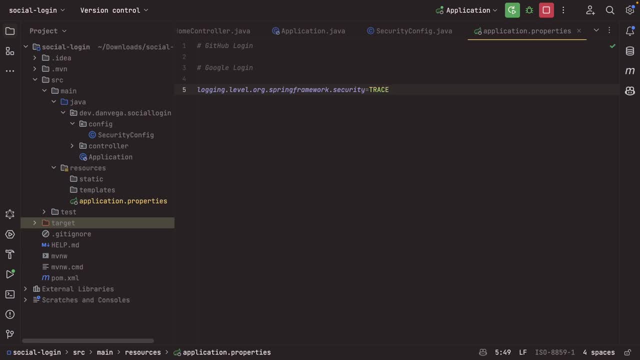 equal to trace. This just gives me some visibility into what's happening in my application, So I like to go ahead and set that first. Now to do GitHub and Google login. I'm going to go ahead and set up GitHub, So let's say I'm going to go to Google or Twitter or whatever You need to create OAuth 2. 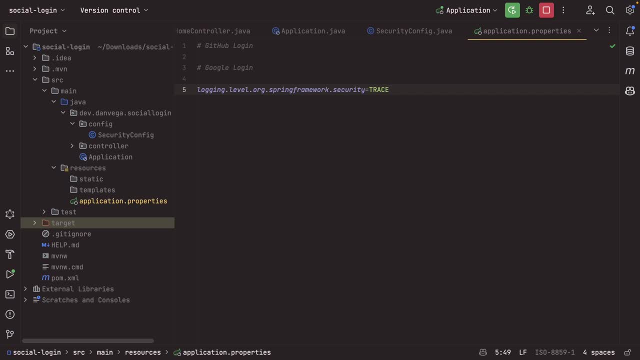 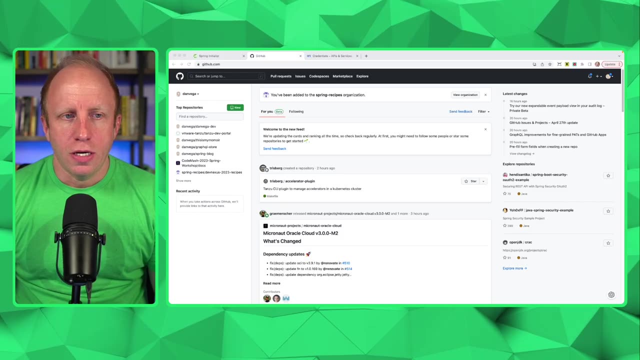 client credentials on their applications, So let's start with one. We're going to head back over to the browser and we'll talk about setting up GitHub first, and then we'll move on to Google. All right, So here I am on my GitHub account. I am going to go over to this little icon here and 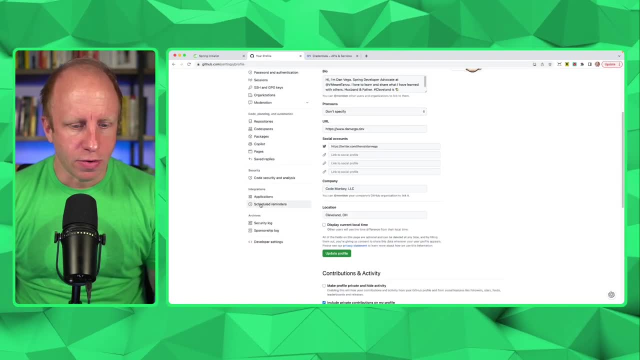 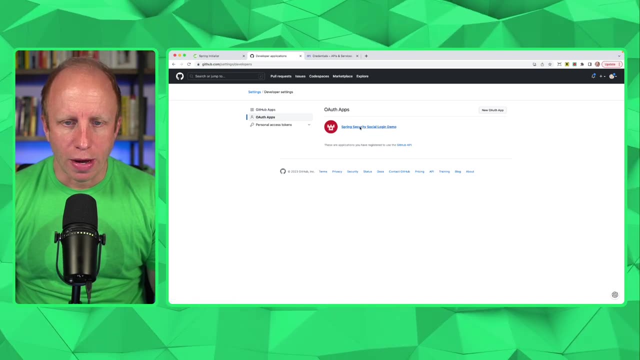 I'm going to go to settings From there. we are going to go all the way down here into developer settings, And we're going to go into developer settings And we're going to go into developer settings And we're going to go into OAuth 2 apps. So you see, I have one here from before. Let's. 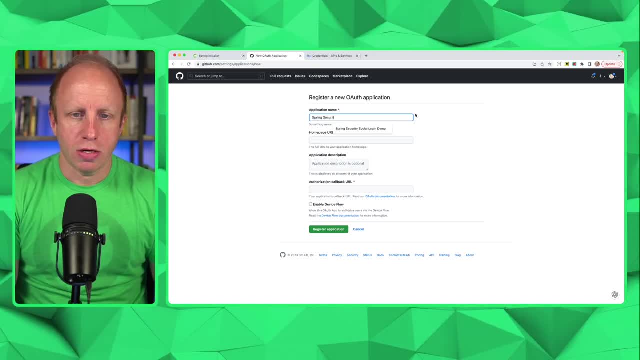 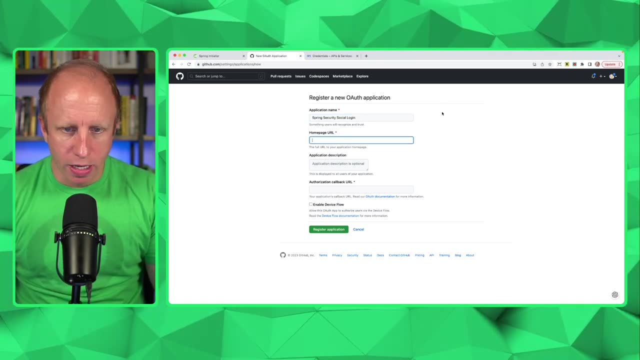 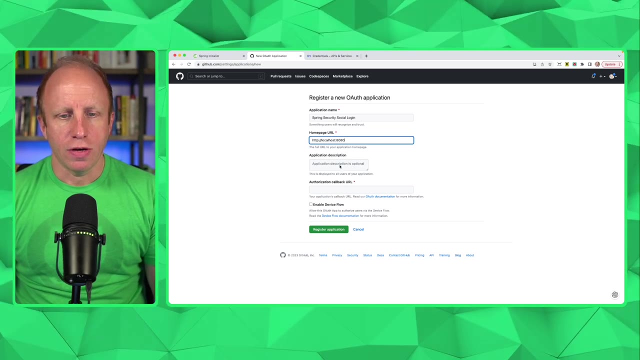 create a new OAuth app. We'll call it Spring Security Social Login. We'll just call it that. And then you need a homepage URL, the full URL to access your application. We'll just say localhost 8080.. You could fill in some information about the description here, And then you need an authorized 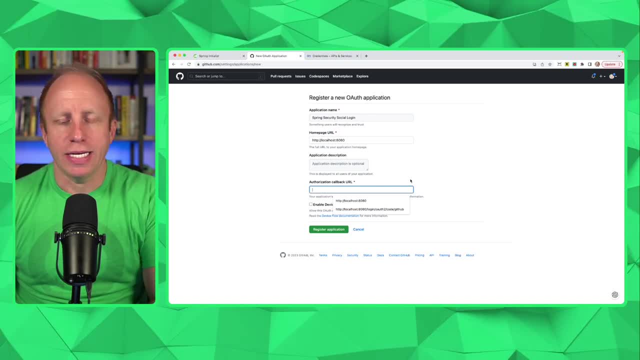 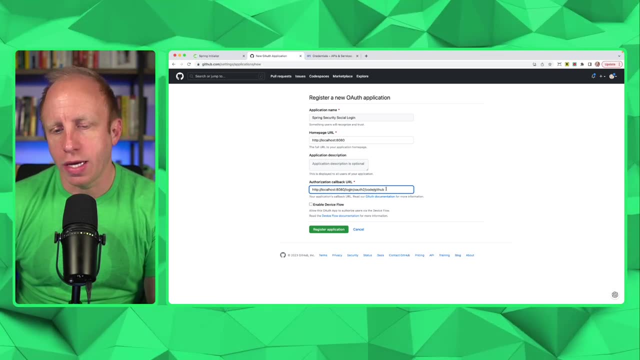 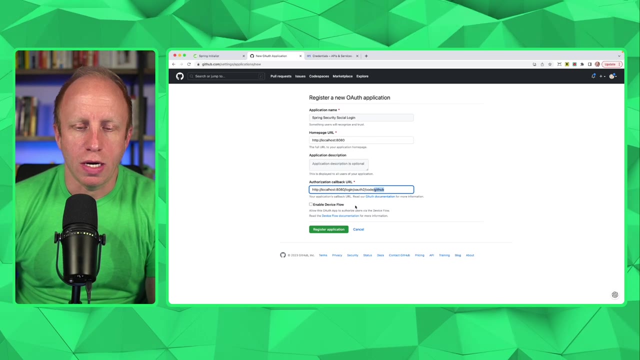 callback URL. So this callback URL, it's something that you would get in the documentation. I actually have it here. localhost 8080 slash login- OAuth 2 code. GitHub Turns out this URL is the same, just whatever. this is going to be replaced with something like Google, So I am using that as my 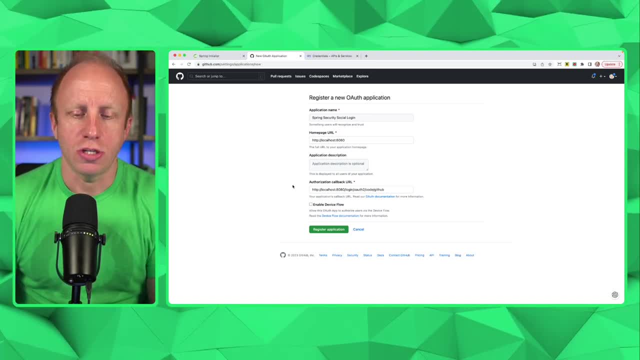 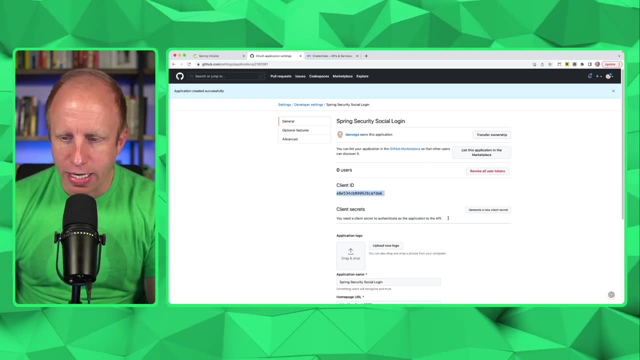 authorization callback URL And then this is going to control the flow in my application. So I'm going to do is register my application And now you can see, I have a client ID and I have to generate a new client ID. So I'm going to go ahead and create a new client ID And then I'm going to 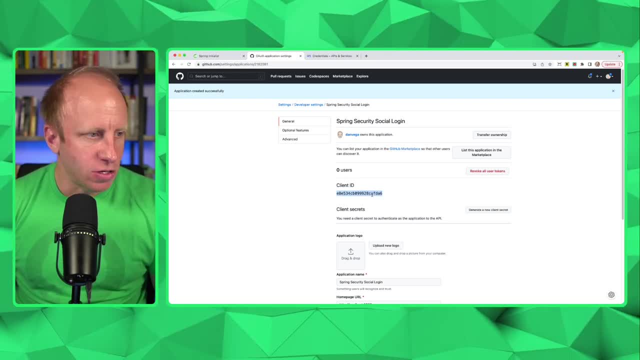 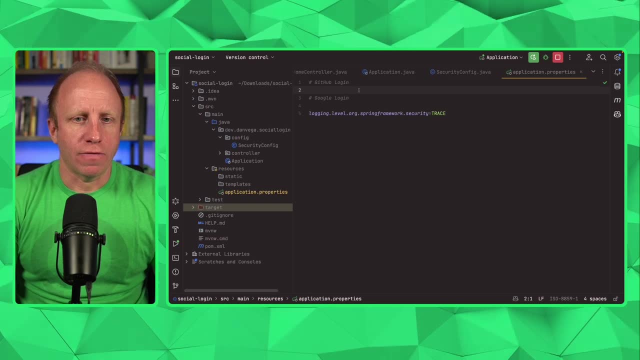 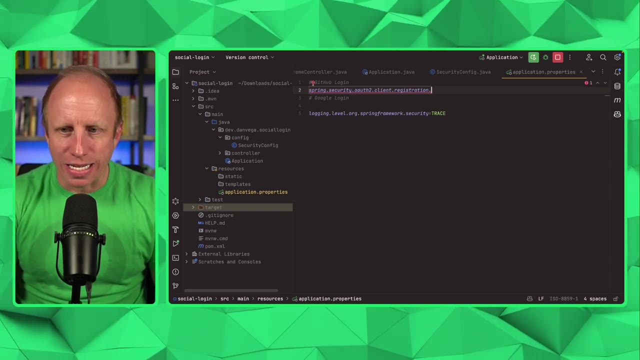 create a secret. Let's take this client ID first and head back over to my applicationproperties. So in here for GitHub login, I'm going to say Spring Security OAuth 2 client registration dot and then the name of the provider. So in this case it's GitHub And I'm going to say the client. 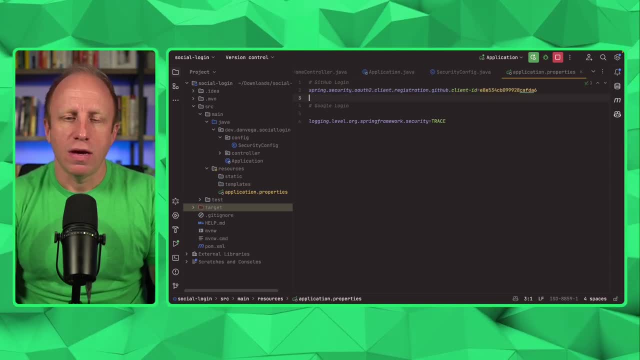 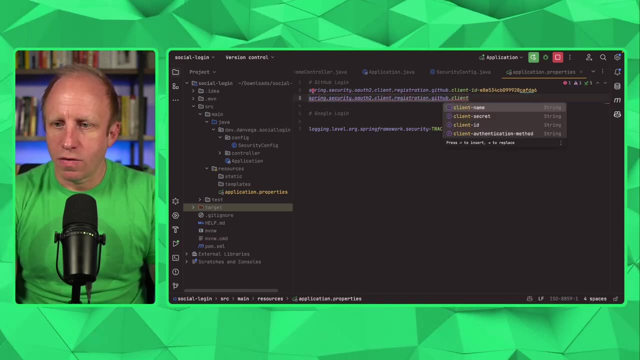 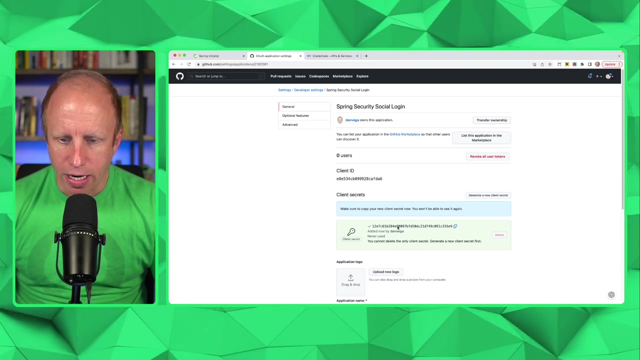 ID is equal to this. All right, So we're going to copy, copy that and then just say the client secret is going to be equal to, and then we'll go back over here, we'll generate a new client secret And I have this. I'm going to copy it Again. I'll go. 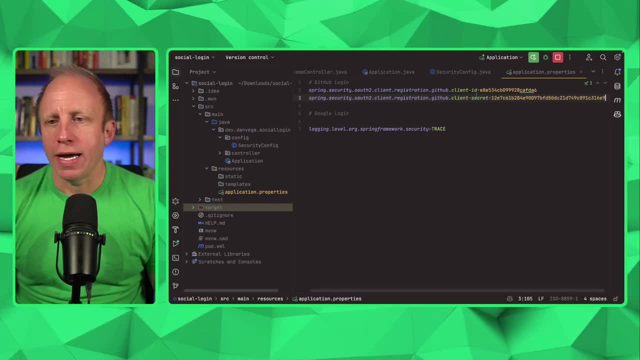 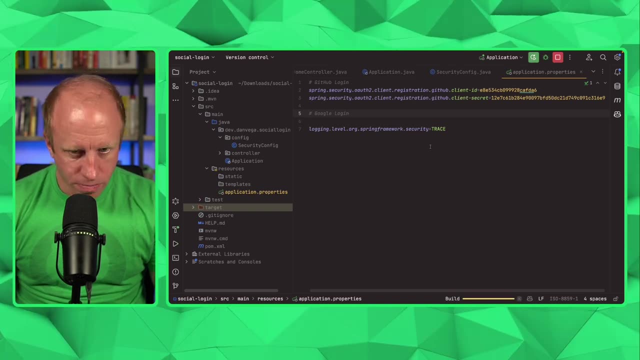 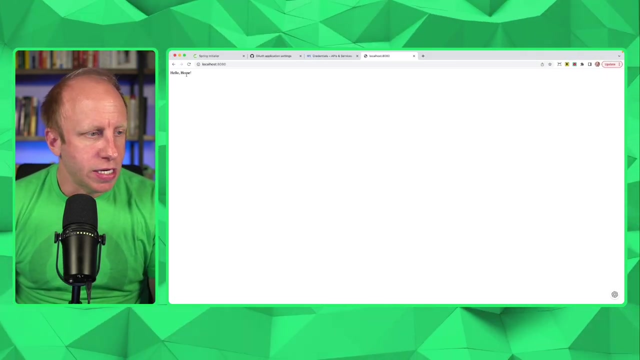 ahead and delete this after the video. But now I have my client ID and my secret, So with that I should be able to go ahead and run the application And if we head back to the browser and if I go to localhost 8080, we get to home. This one is allowing anyone. 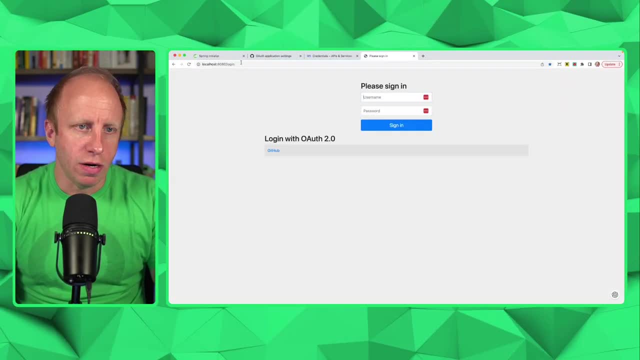 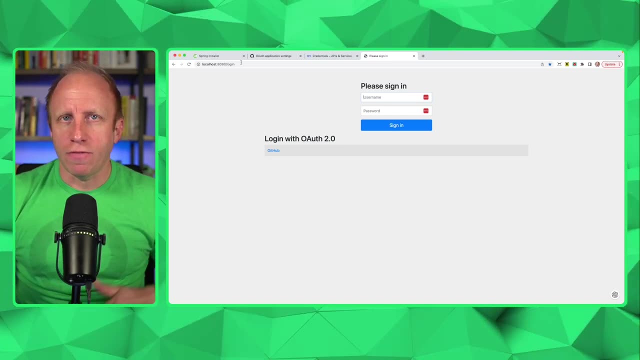 without authentication to get to it. But if we go to slash secured, it's going to ask us to log in. So, again, we provided a form login as one of the options. If I didn't provide the form login and I only had one OAuth 2 provider, in this case GitHub- it would automatically forward. 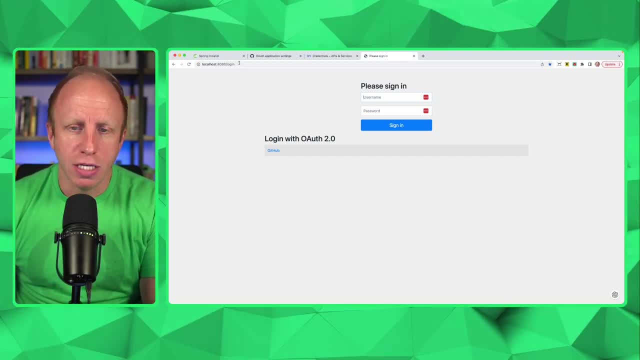 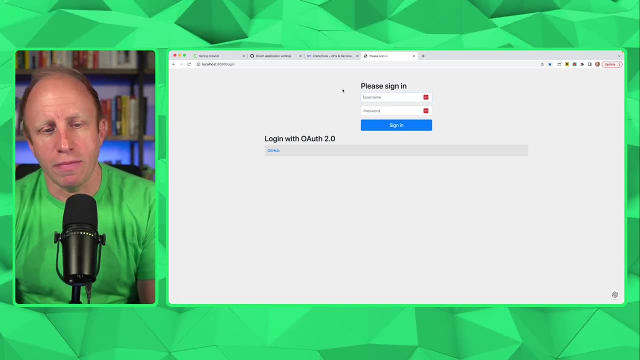 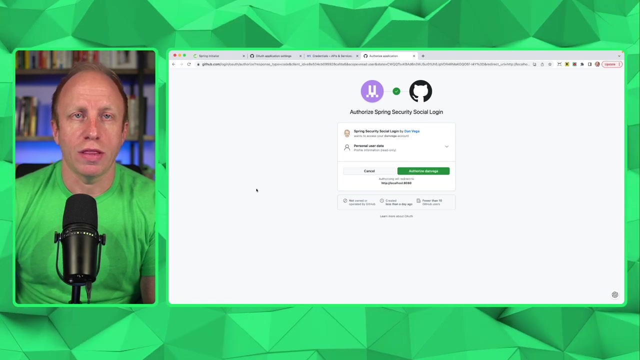 to that GitHub login. I'm having both options here, So that's why it shows me the form That comes out of the box with Spring Security, And then it actually sets up the links for you as well for any of the OAuth 2 providers. So in this case, it's GitHub I need to log in with. 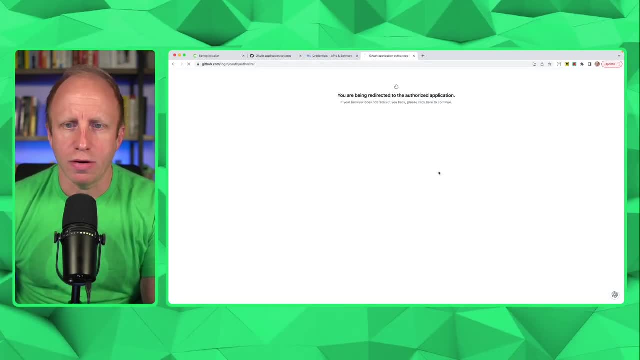 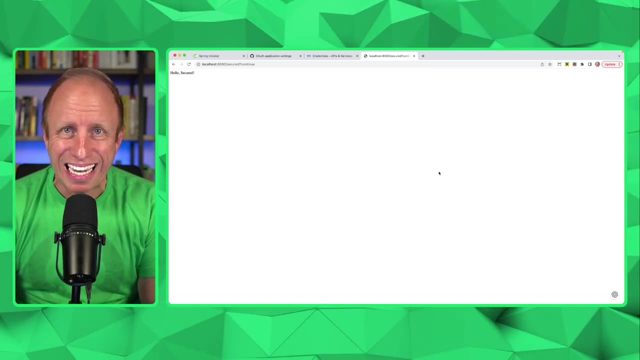 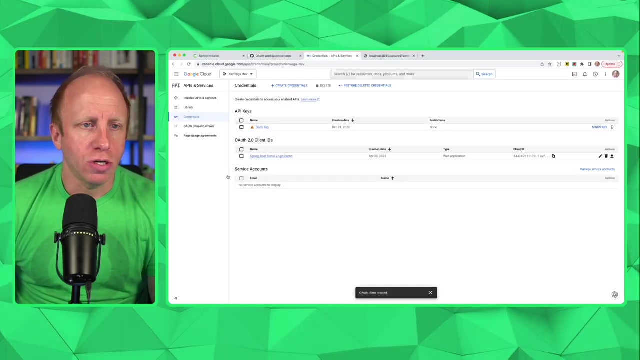 GitHub to view the secured page. I'm going to say, okay, go ahead and authorize that, And I'm forward on to the secured route. So great, That was it. That's that easy to get going. What I want to do now is do the same for Google. So, Google, you will want to go over to. 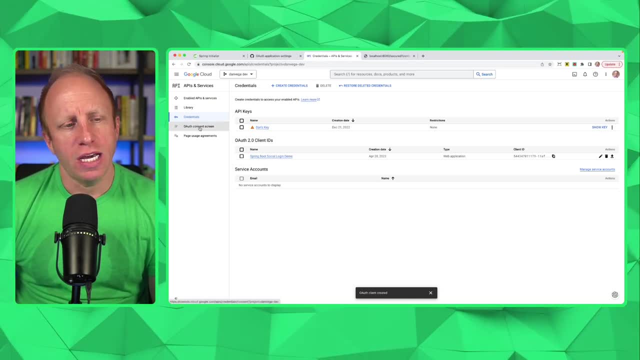 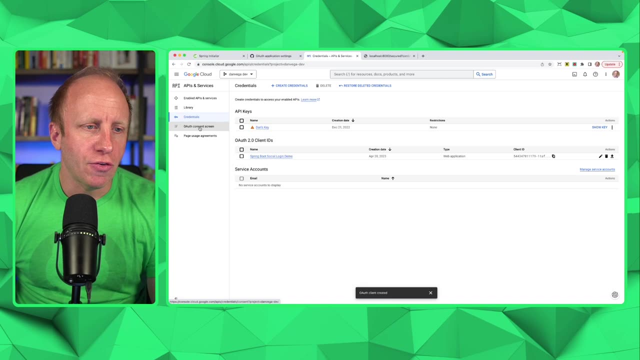 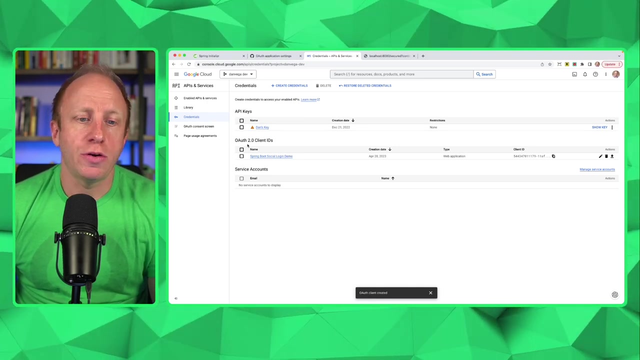 councilcloudgoogle. I will say it was a little confusing. You have to set up the OAuth 2 consent screen first. If you've never done this, you need to do that first. Once you're done there, you can go ahead and go to the credentials area and then create a OAuth 2 client ID. 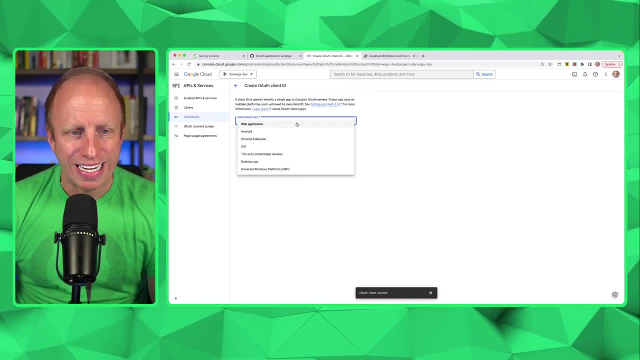 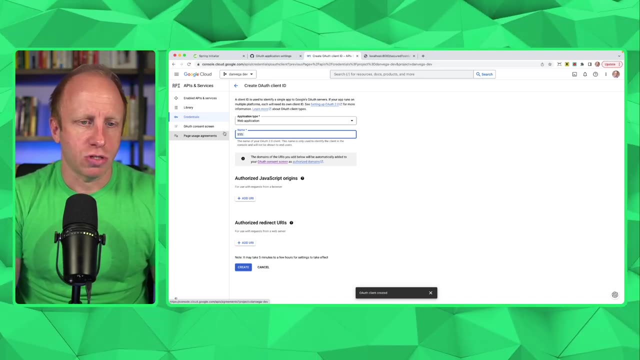 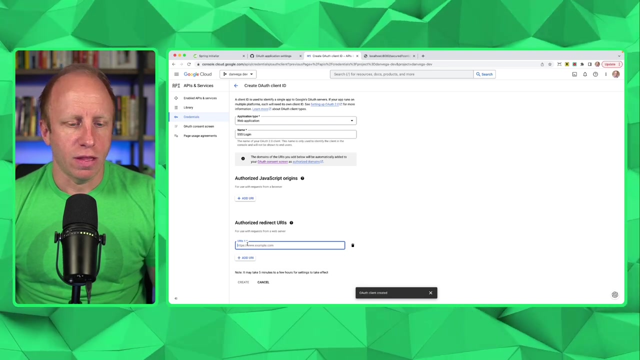 So we're going to create credentials, OAuth 2 client ID. You're going to pick a web application and then you're going to give it a name- So Spring Security, social login- And then you need to add an authorized redirect URI. So, again, this is going to be the same as 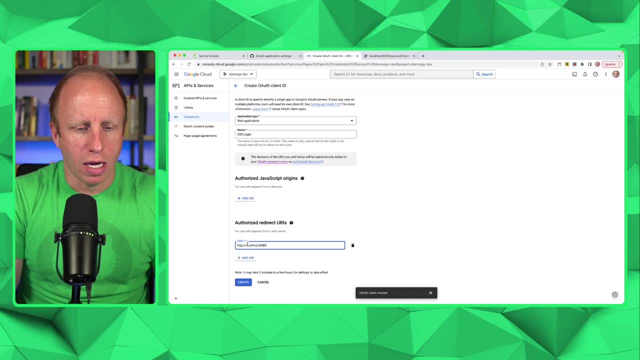 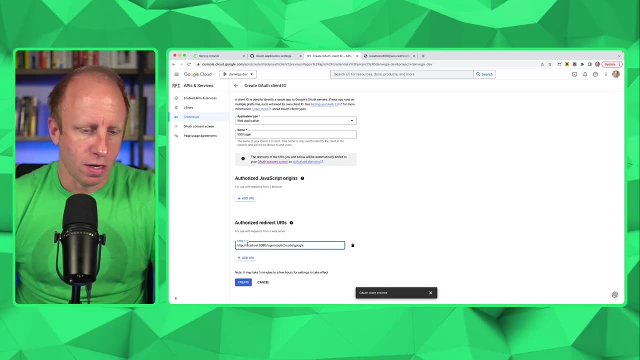 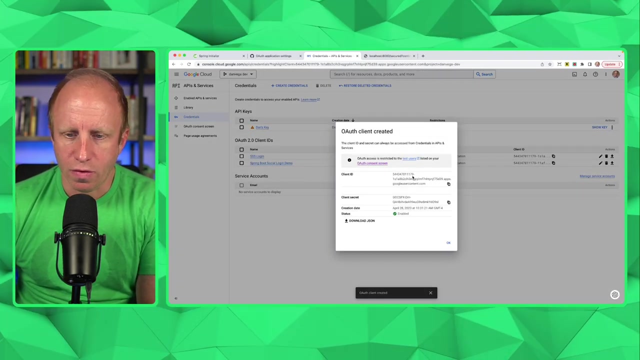 before, which was localhost, 8080, slash, login, slash, OAuth 2, slash code, and now Google. So we're going to add that URI and then create, And then what it's going to do is it's going to give us that client ID and that client secret. So I'm going to head over to here. 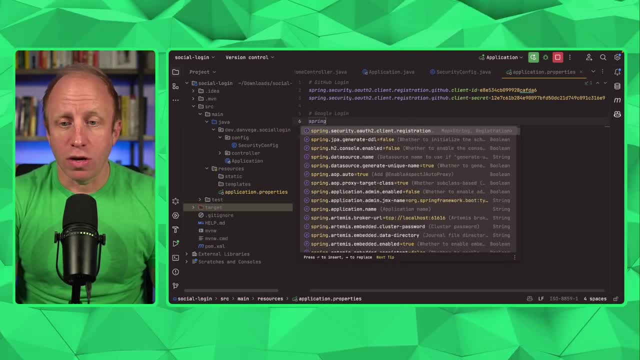 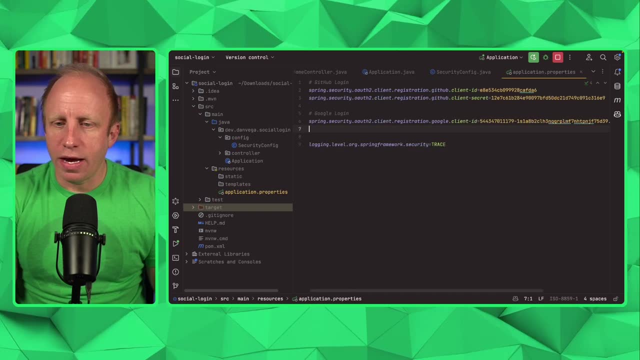 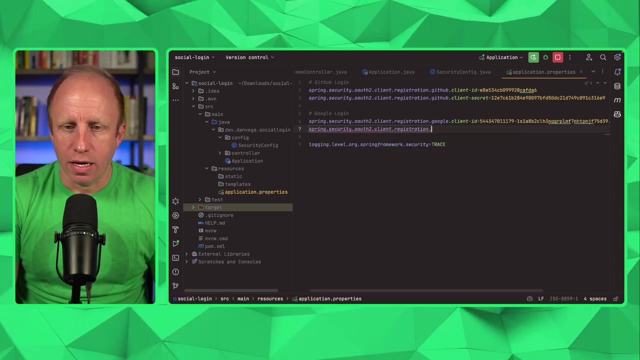 And I'm going to say the same thing. So Spring security, OAuth 2 client registration, googleclient ID, And then we'll pass that in, And then let's head back over here and copy the secret and Spring OAuth 2 client registration, Google and the client secret. 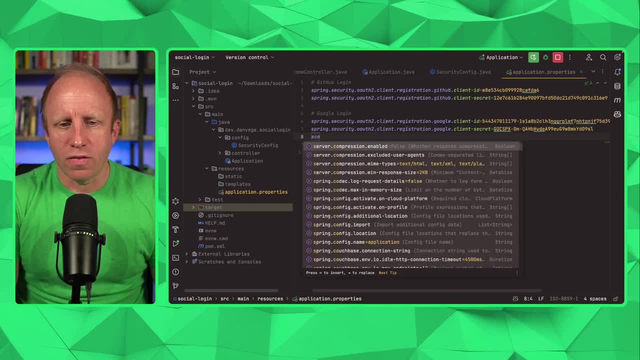 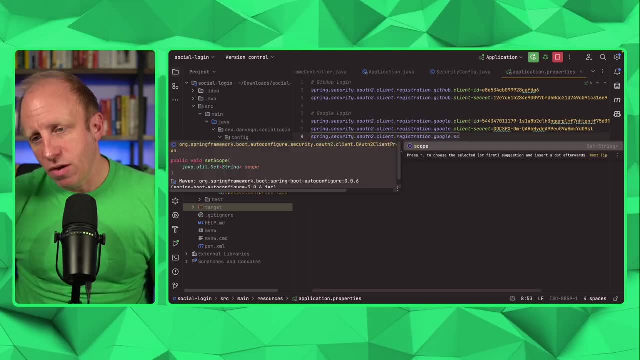 So there's some other things that you can configure in here. There is like: so, if I'm in Spring Security, OAuth 2 registrationgooglescope. So there are things like scope, where you can say, like what is the available scope of this OAuth 2 application, Like what information? 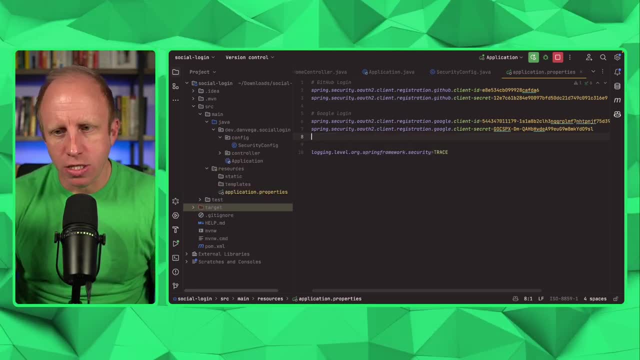 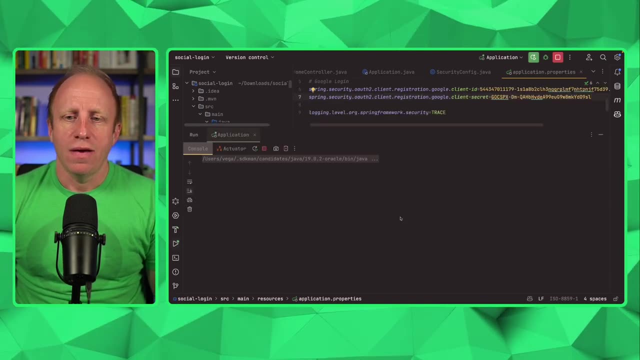 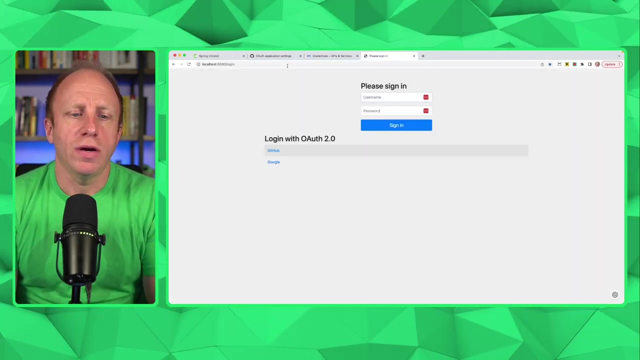 do we want to access. So go ahead and read the documentation If you want to dig down and figure out what else you can configure here. but that is it for this. I'm going to go ahead and restart this and we will see that if we go to localhost, 8080, slash secured. we are now 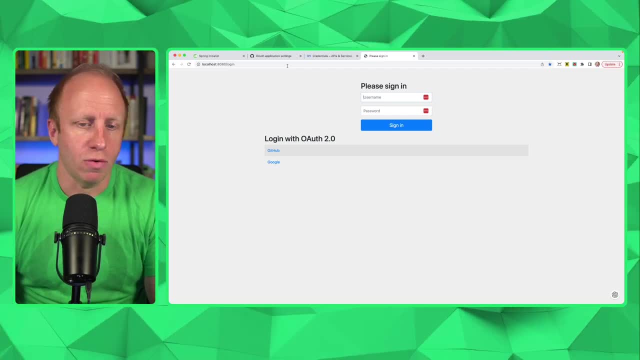 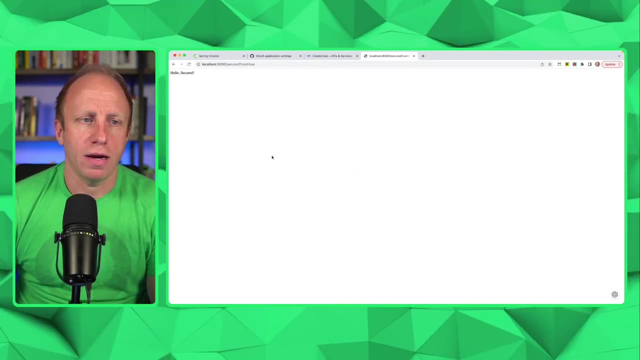 given two options. So we can log in with GitHub or we can log in with Google. So now I'm going to try Google. Here are my different options for my Google account. I'm going to sign in with that And, as you can see, I am taken to the secured page. All right, thanks for sticking around to. 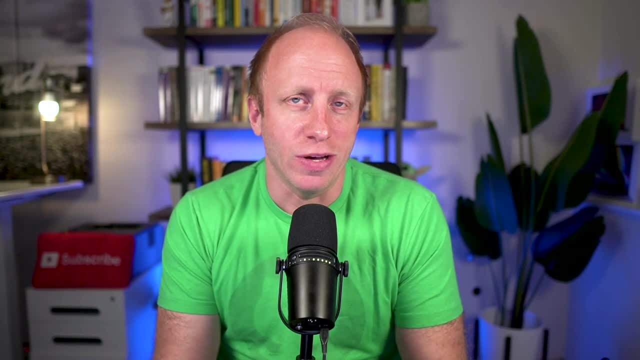 the end of that tutorial. It was a short one, but a sweet one. I know a lot of you were asking me about how to do that. Obviously, this is just kind of one piece of the puzzle when it comes to security and OAuth and open ID. there's a lot to learn, Uh, but this is a good way to help you. 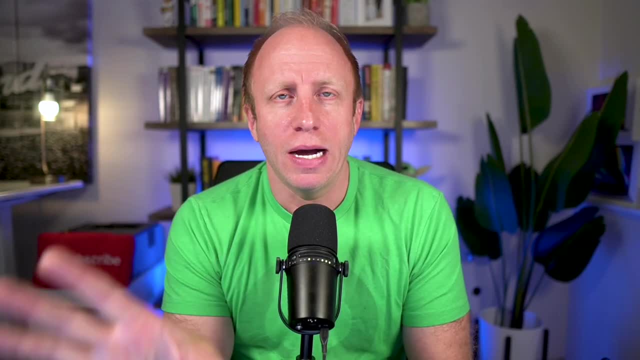 I know a lot of you were asking me about how to do that. Obviously, this is just kind of one piece of the puzzle. when it comes to security and OAuth and open ID, There's a lot to learn. Uh, but this is a. There's a lot to learn, but this is extremely easy to set up in Spring Boot and Spring Security. 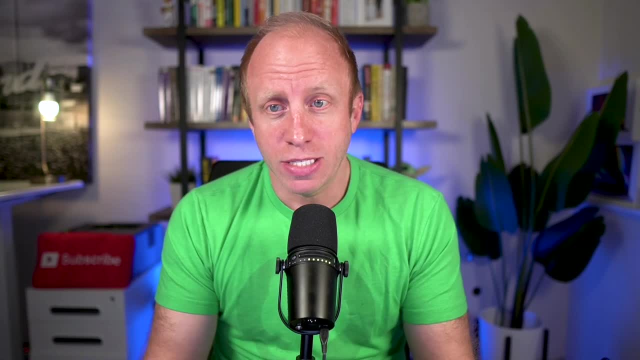 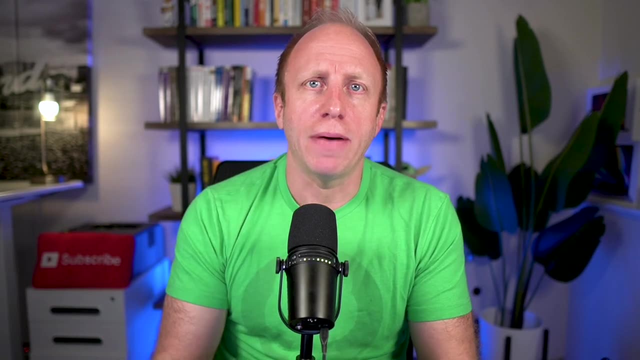 so I just wanted to kind of walk you through that. Now, something else I've been asked about and I'm interested to hear from you to see if it's something you're interested in. we get that out-of-the-box form login that. 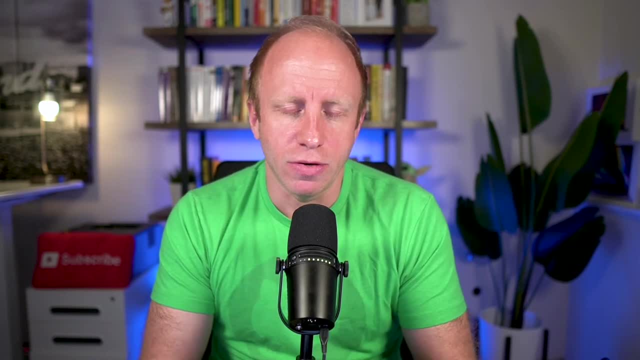 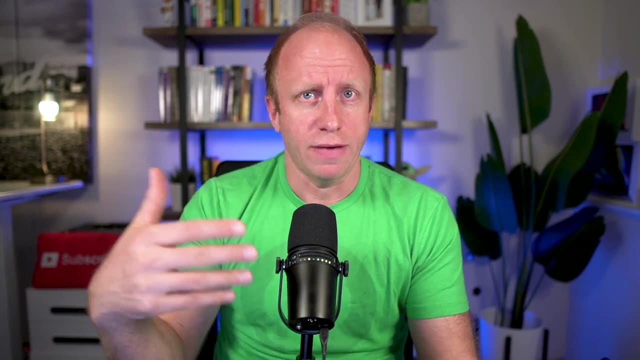 out-of-the-box ability to log in with GitHub and Google. but what if you wanted to customize that page? You can do it. You can override the login page. You can kind of set that up in Spring Security and maybe you're interested in customizing. 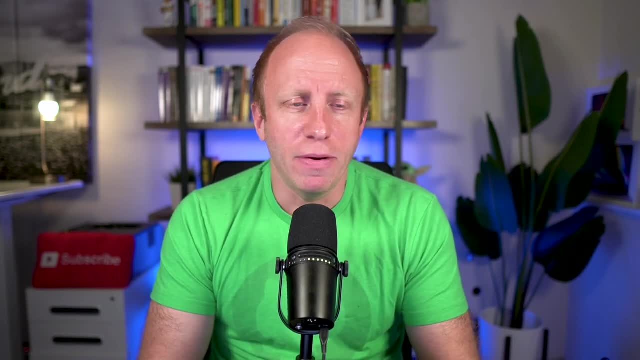 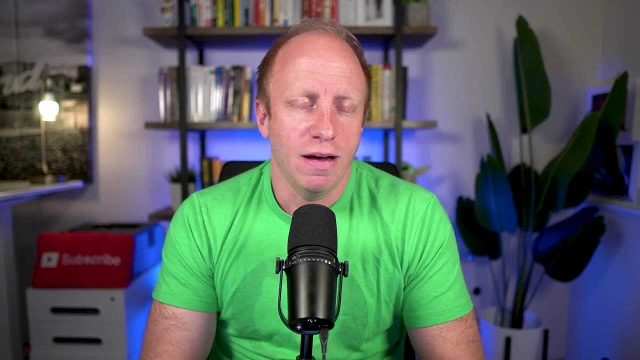 that. If you'd like a tutorial on that, let me know. I'm a big fan of creating front ends, so I would create. you could do this in like TimeWave, but I would use something like Vite and Vue to create that and something like. 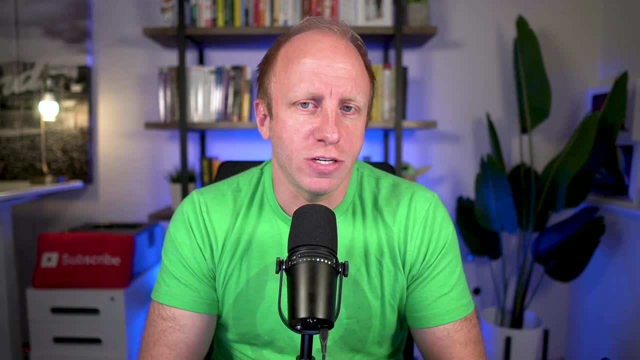 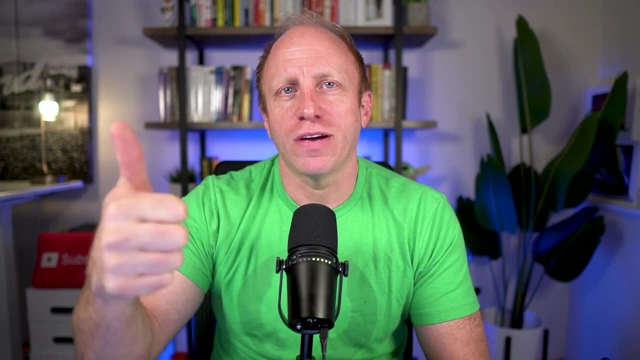 Tailwind to style it up. so I think that would be a fun tutorial. If you're interested in something like that, let me know. But what about this one? If you found some value in this tutorial? If you found some value in this tutorial, friends, do me a favor, give me a thumbs. up, subscribe to the channel and, as always, happy coding. 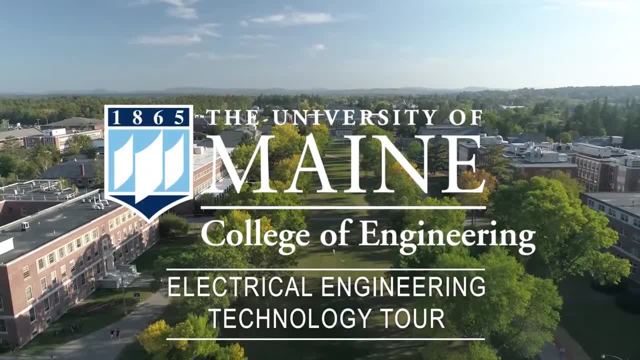 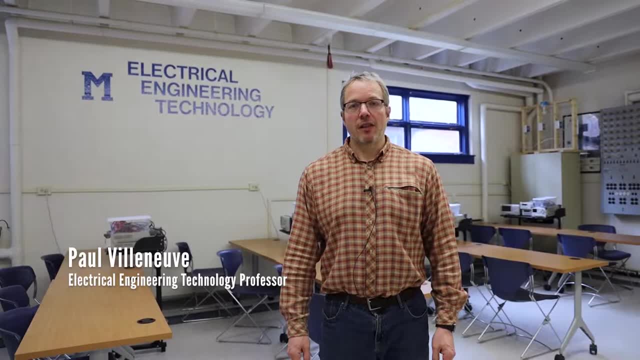 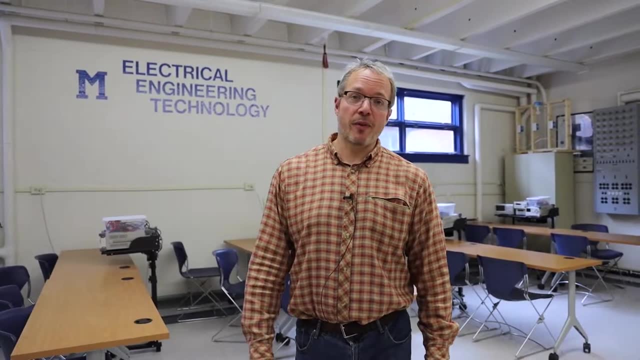 So welcome. my name is Paul Villeneuve, and today we're going to give you a little bit of a tour of the electrical engineering technology labs that we have located in Barrows Hall. I am an associate- actually I'm a full professor- and have been with electrical engineering. 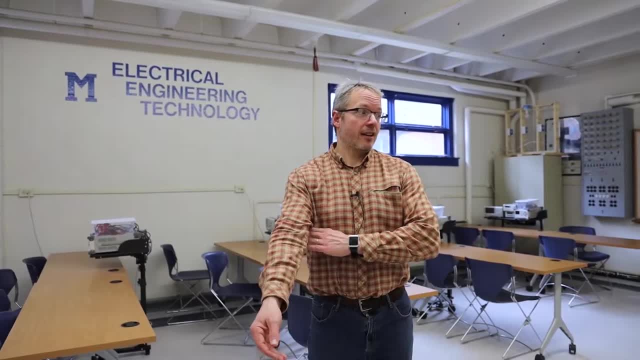 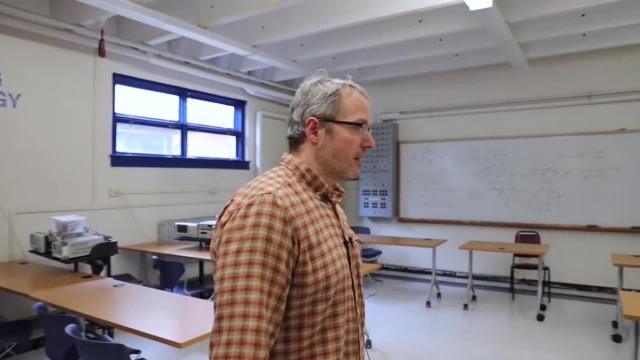 technology for 17 years. I'm also a graduate of UMaine and actually took a number of courses in the electrical engineering technology program. So if you decide to start in our program, you'll spend a fair amount of time, especially in your first year, in this room. 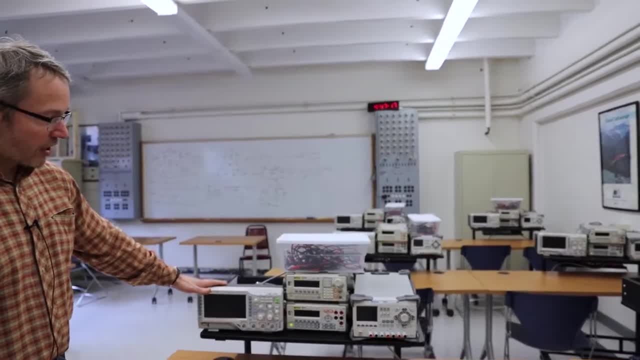 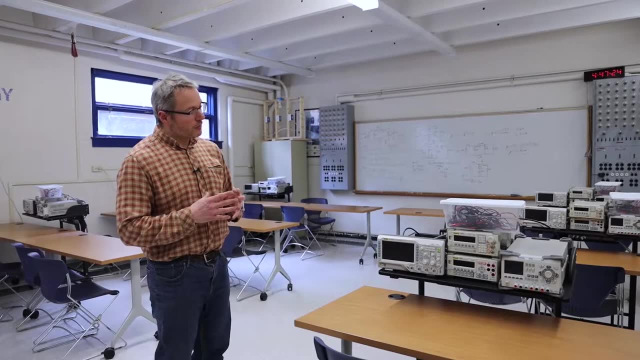 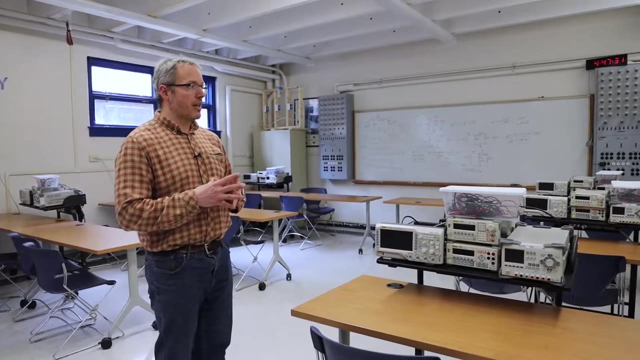 This is the analog components analog electronics lab, where we get to build circuits, small scale breadboard circuits, to sort of verify fundamentals and prove that they actually match the equations that you'll be learning in class. So each station we currently have 10 and we'll be upgrading those to 12.. 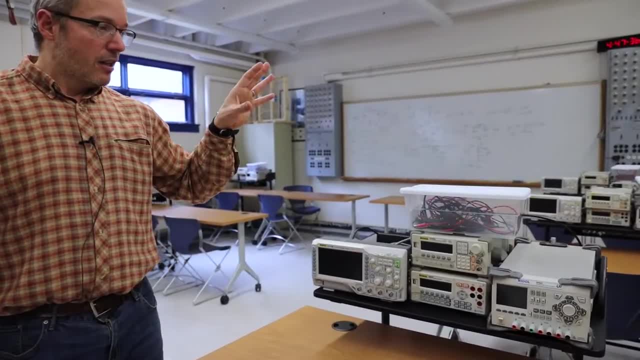 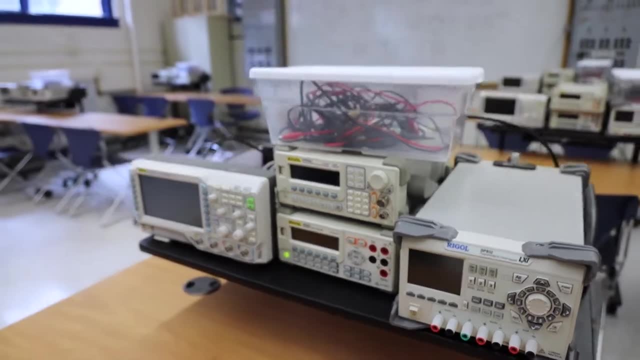 Each station has a number of circuits that we're going to be upgrading to 12.. Each station is exactly the same. We have some DC power supplies, we have some AC power supplies, which are called function generators, we have oscilloscopes and we have multimeters, along with a number. 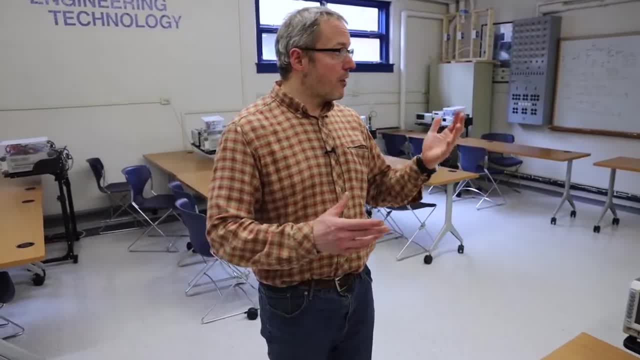 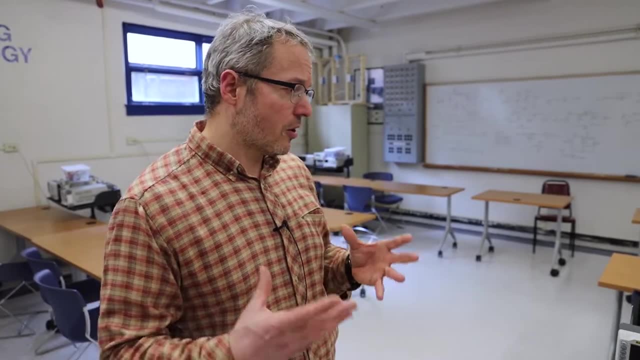 of cables and whatnot per station. We do have components in some of the back cabinets and it allows us again to just really kind of emphasize and build actual circuits. So in terms of you know, one of the distinctives of engineering technology is really getting 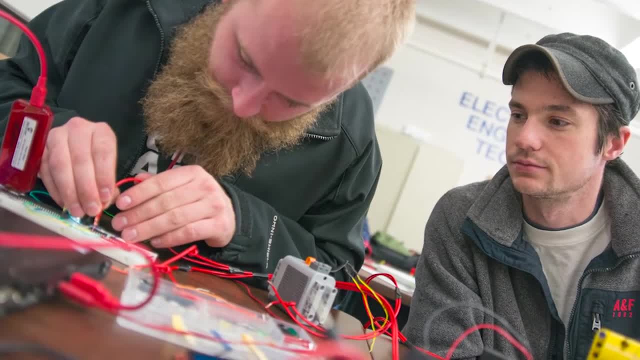 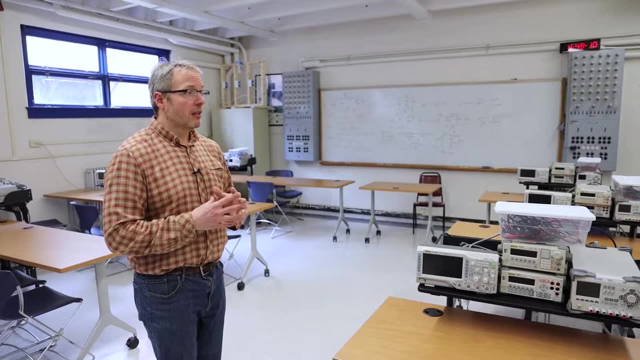 a good feel for what's happening from a practical perspective and building physical circuits. And so this lab- we get you to build a lot of circuits and demonstrate that. We spend three to four classes utilizing this lab to really demonstrate and see what's going. 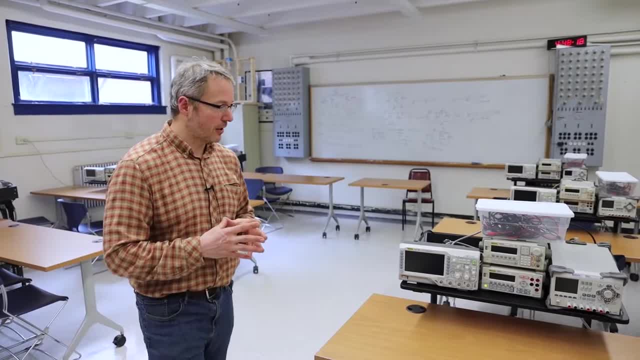 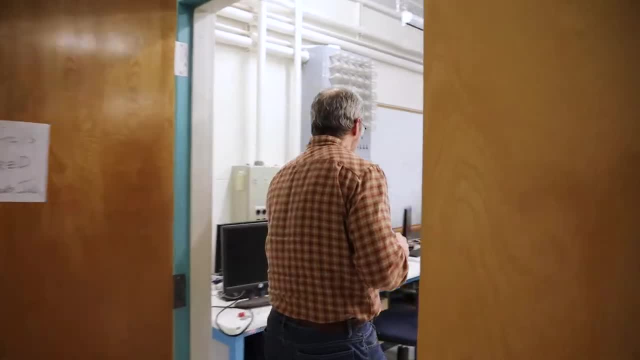 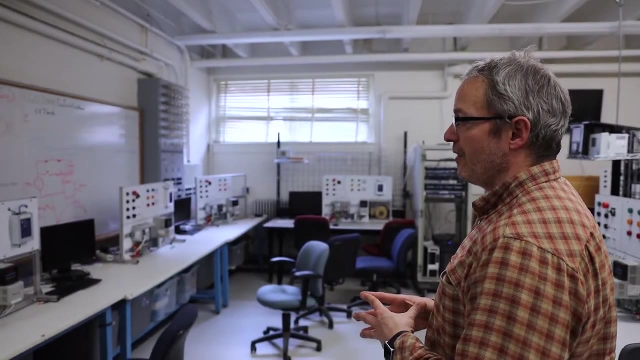 on in these particular electrical circuits. So let's move on to our next lab. Next lab we'll be looking at is for PLCs, essentially industrial automation. So if you were to go to a paper mill or a processing facility, you'll find these type of components.